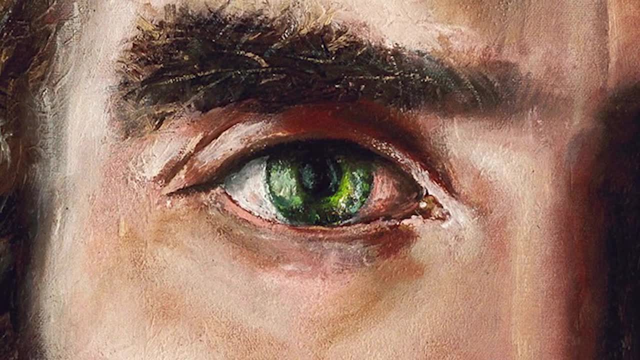 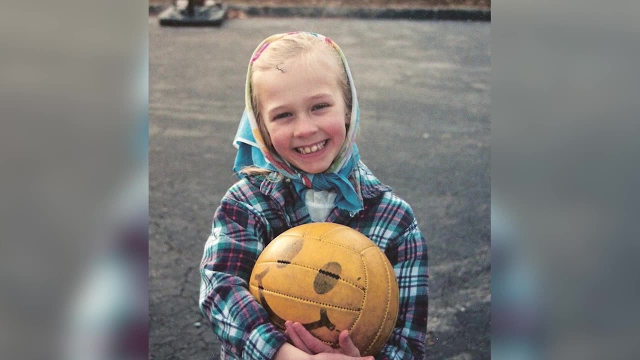 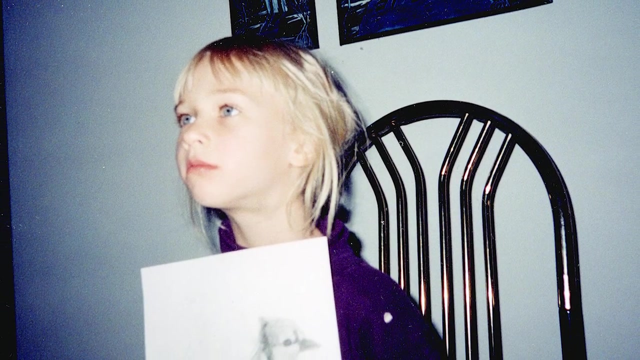 An eight-year-old once painted a picture that eventually sold for almost a million dollars. Around the age of four, Akiana Kramarik began experiencing visions which she couldn't put into words, so she started drawing them. Her parents noticed right away that she was highly gifted. 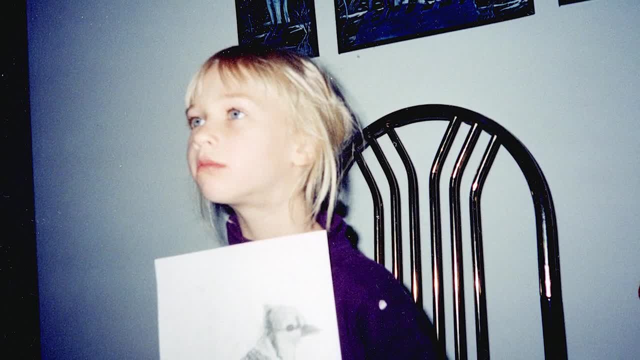 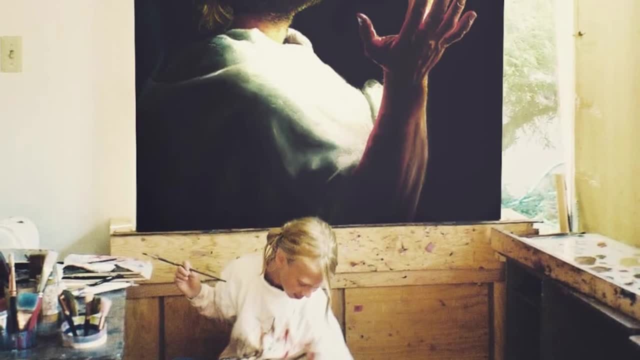 so they provided her with all the material she needed and allowed her to focus on this completely. By the time she was five, her sketches looked like an adult artist. By the time she was six, she started painting. By the time she was seven, her paintings were amazing. 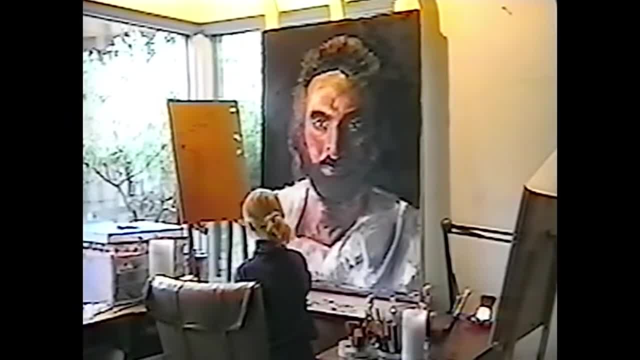 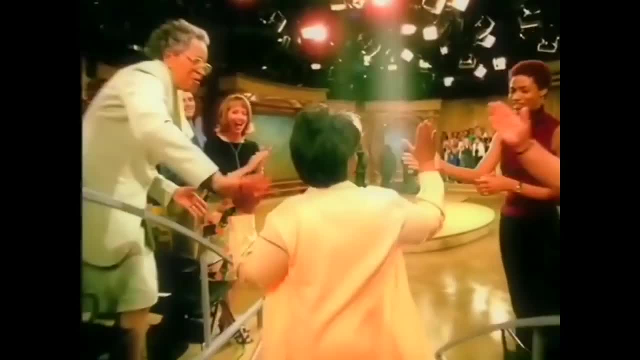 At the age of eight, she painted her famous Prince of Peace, which was an image that had come to her in a vision. By the time Akiana was nine, Oprah Winfrey caught wind of her. Our next guest is already earning $25,000 for her work, and she's only nine. 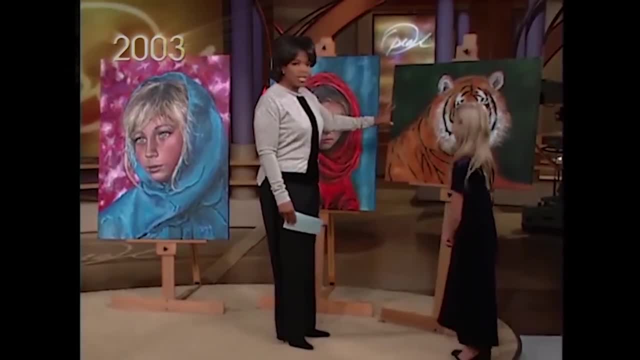 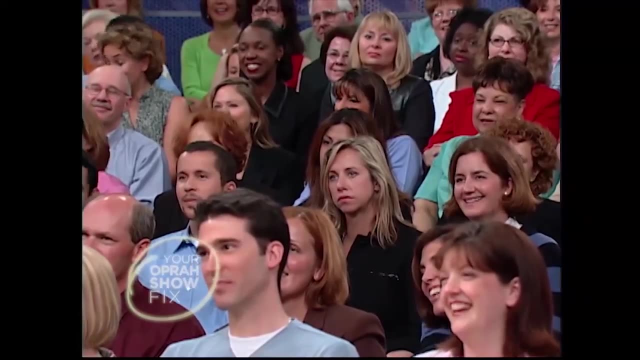 And Oprah did what Oprah does. She lifted her up for the whole world to see, exalting her to fame. The world witnessed Akiana. The world saw her in her work and realized, together and in an instant, that we were in the presence of genius. 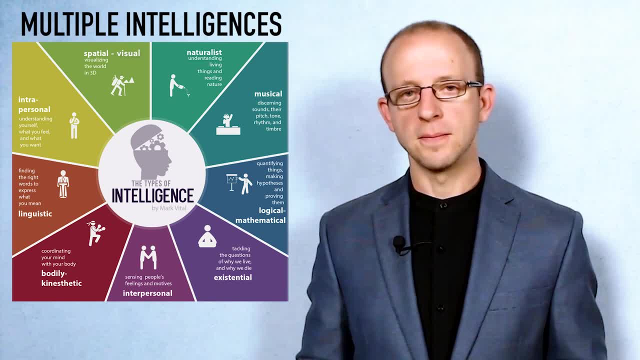 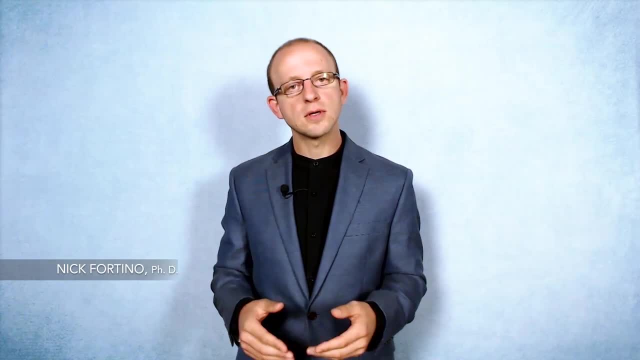 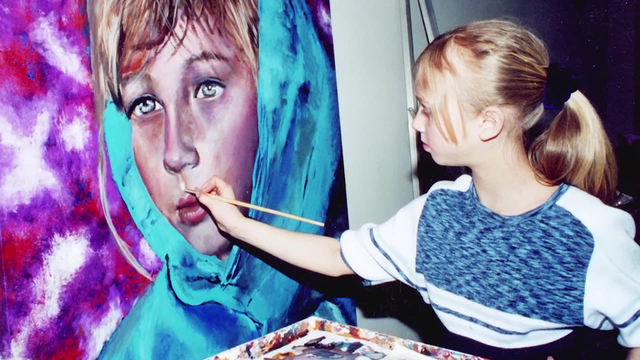 In the multiple intelligences theory, there's a set of criteria that each intelligence has to meet to be considered an intelligence, one of which is that there must be examples of geniuses, of people who exhibit this intelligence to an extreme degree. Akiana Kramarik is in doubt. 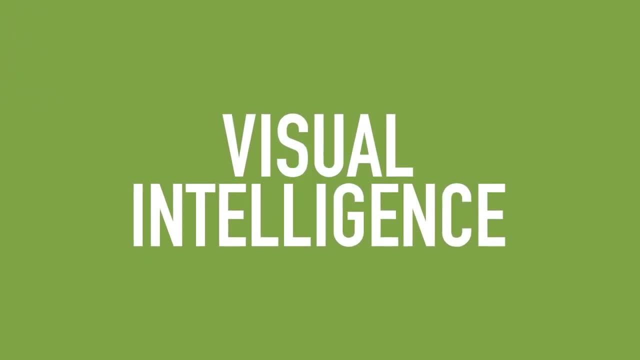 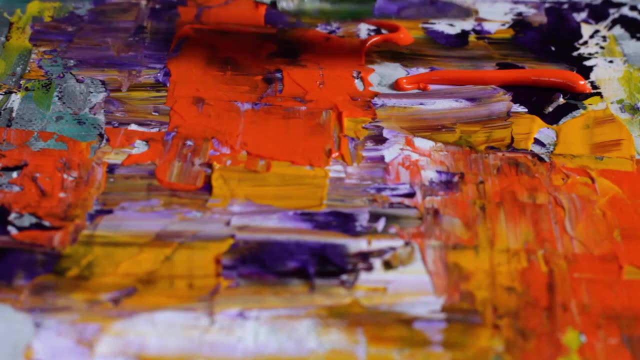 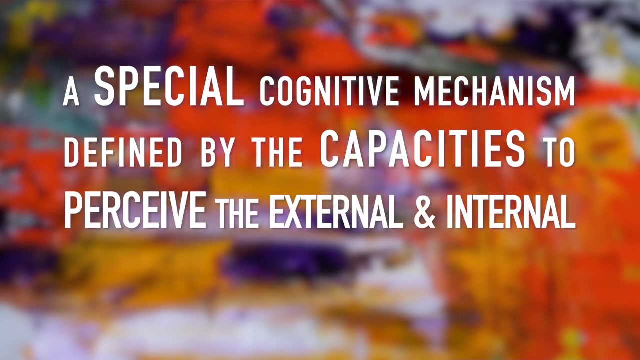 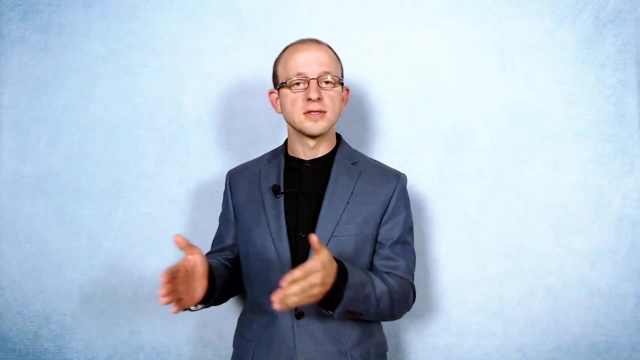 But there is a genius of visual intelligence. Howard Gardner, the pioneer of this theory of multiple intelligences, described this intelligence as a special cognitive mechanism defined by the capacities to perceive the external and internal visual world vividly, to perform modifications on the initial perception. 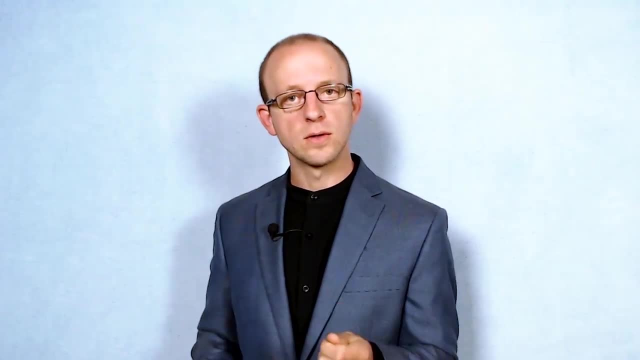 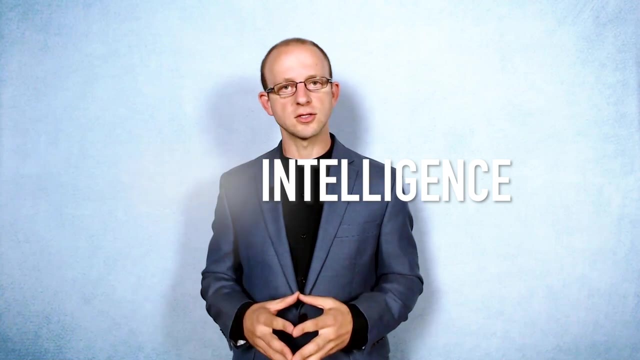 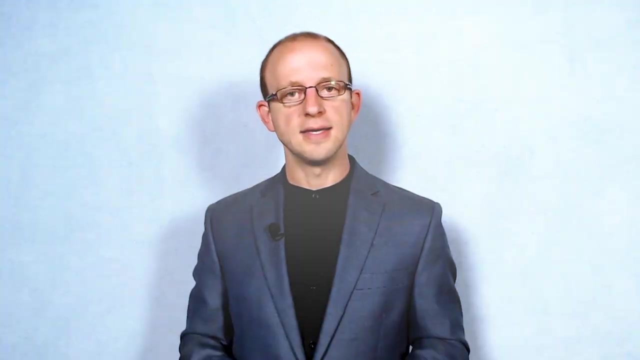 and to recreate aspects of one's visual experience. And so a quick note on the term visual intelligence: it's often used interchangeably with spatial intelligence, And Howard Gardner preferred spatial intelligence because it didn't leave out blind people And he argued that blind people can be visually intelligent. 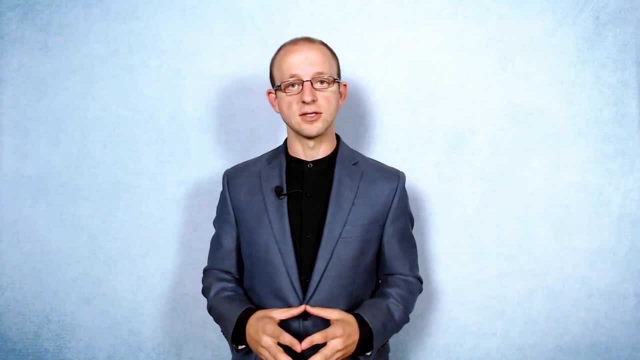 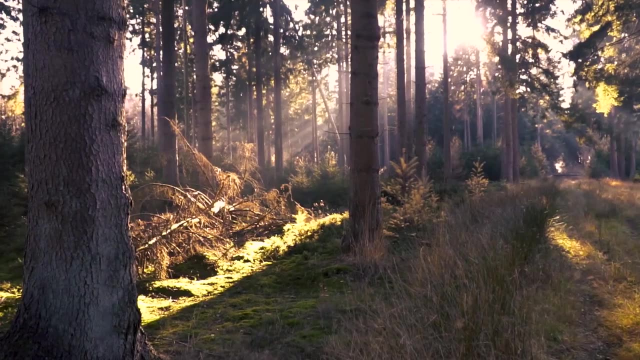 in the same way that a deaf person can be musically intelligent. So we can use the words interchangeably. but visual intelligence is nice and accurate because it's referring to the way in which a person can process visual information that is coming in the form of images. 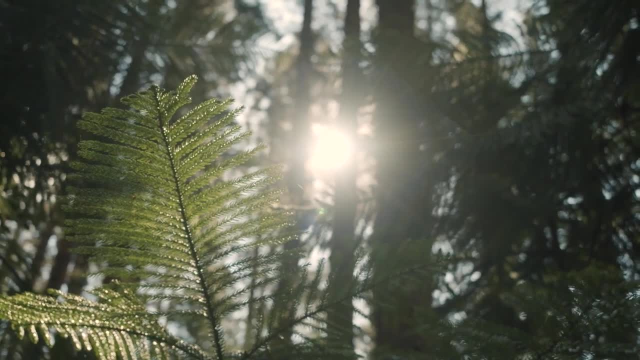 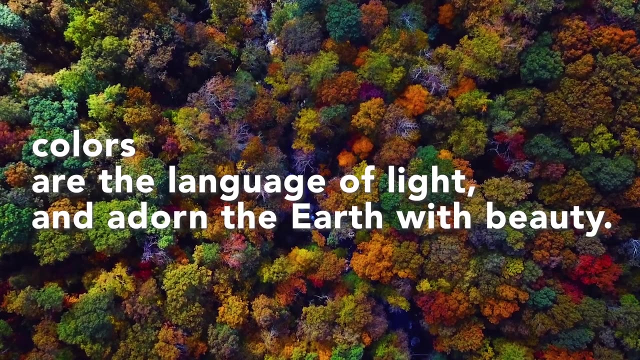 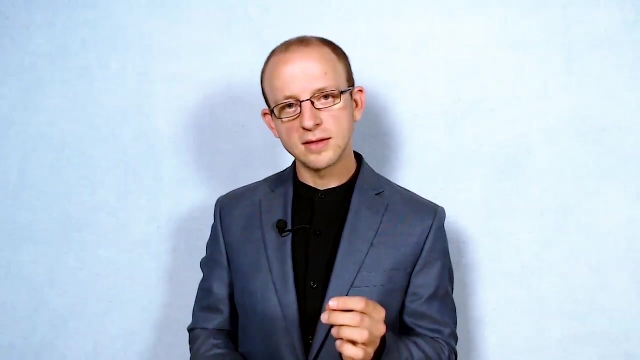 We're talking about the world of light. All visual input colors, the poet John O'Donohue said, are the language of light and adorn the earth with beauty. Put simply, visually intelligent people know what looks good. They speak the language of light. 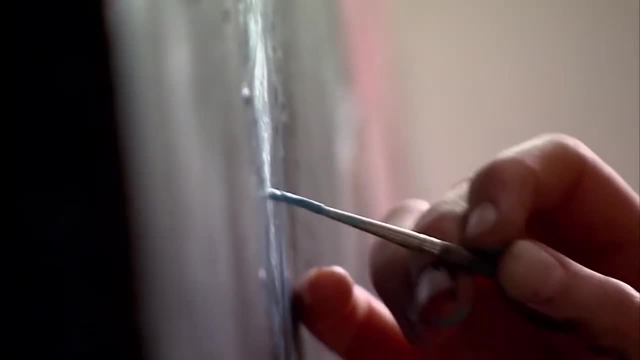 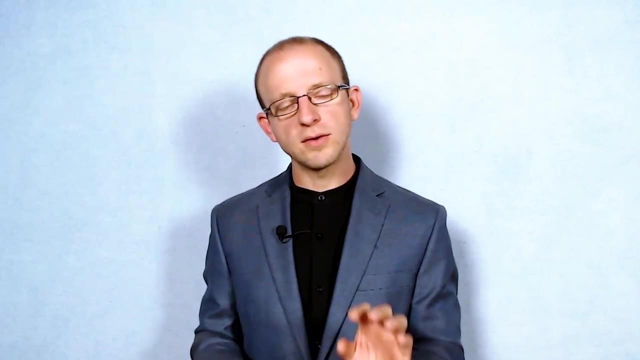 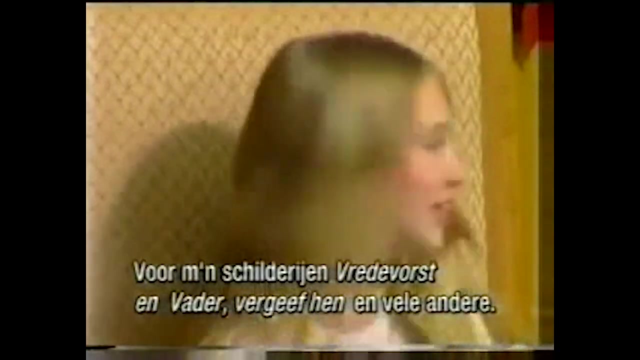 It also applies not only to the external world of light but the inner world of visions and images and memories and literally anything you can experience internally that manifests in the form of an image, Visions of paintings, the Prince of Peace and the Father Forgiven. 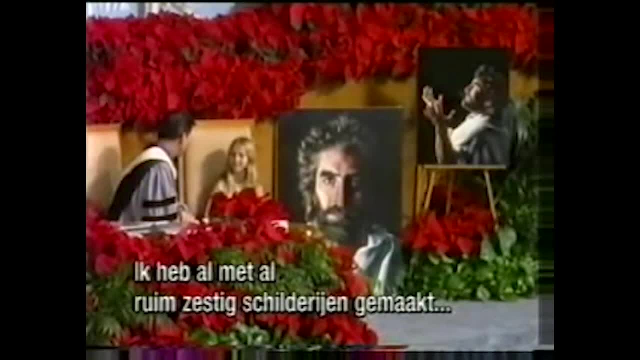 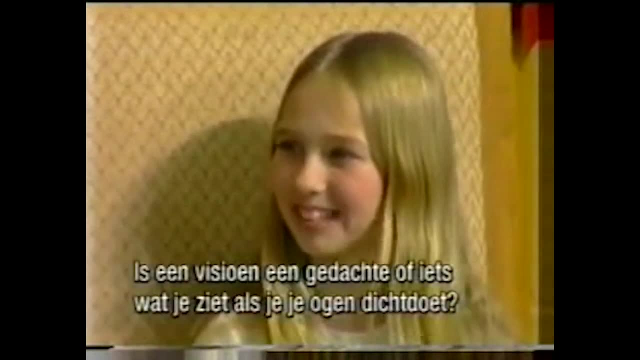 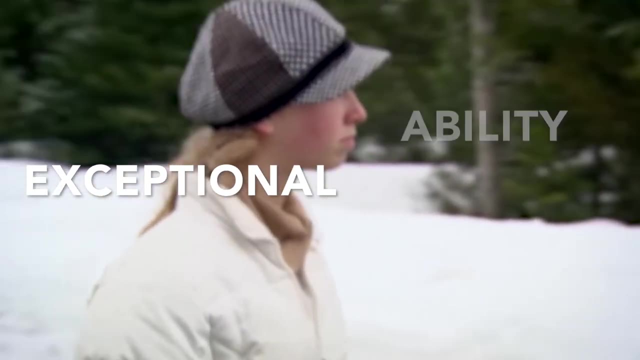 and many, many others. all those are visions. I just forget them. The way I can remember them is to write them or to paint them. So what exactly do we mean by genius? Geniuses possess this trifecta where they have exceptional ability. 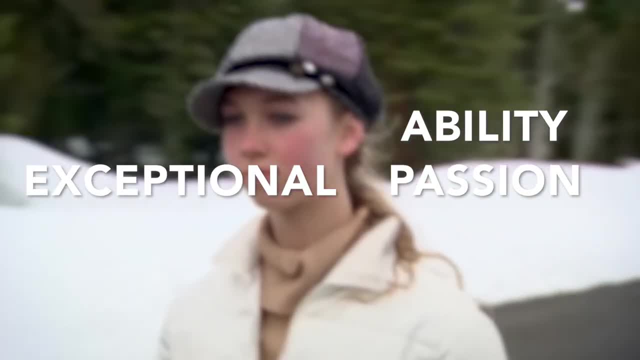 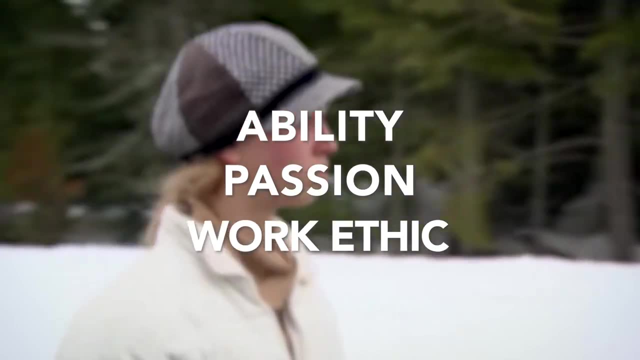 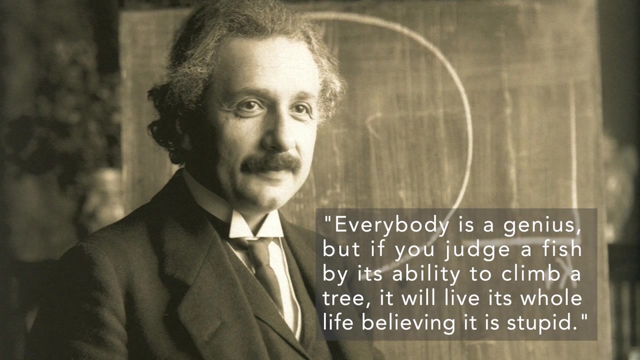 exceptional passion and exceptional work ethic, Exceptional meaning for each of those three areas. They are in the top percentile And let's remember that, as Albert Einstein said, everybody is a genius. But if you judge a fish by its ability to climb a tree, 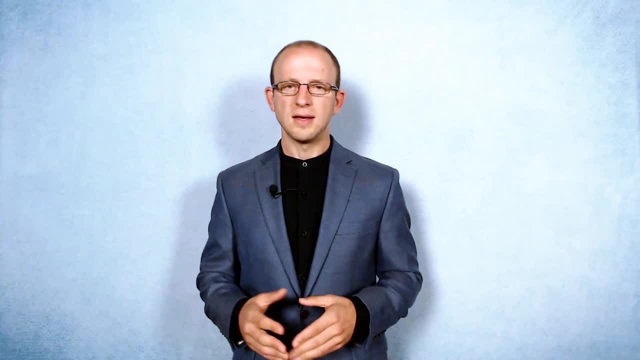 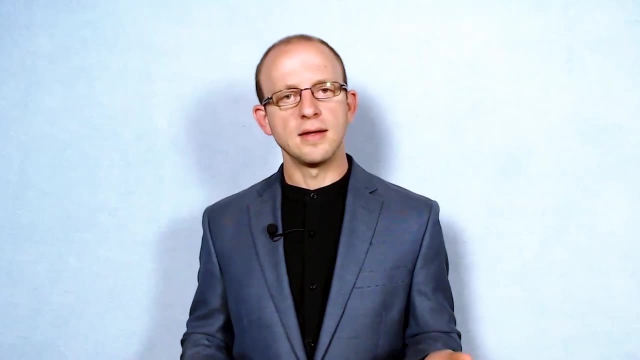 it will live its whole life. believing it is stupid. And it's not just to make you feel good, It's to make you feel better type of affirmation to say that you really are a genius. It's true that when an individual finds what they are good at, 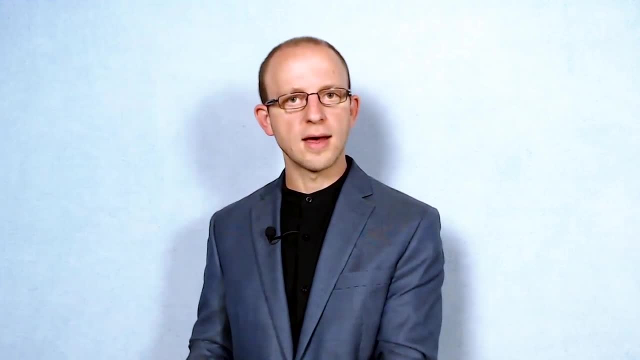 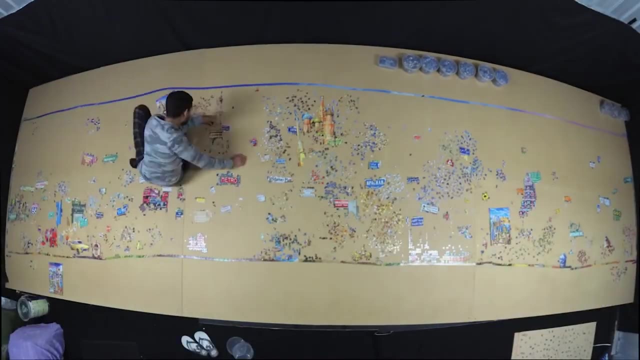 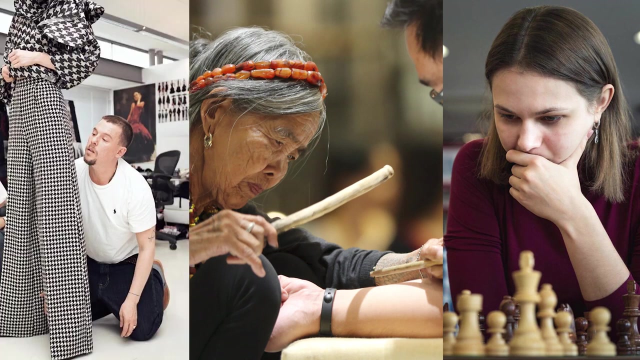 and then they have the opportunity to develop what they are good at. like a fish that finds water, they will thrive. Visual intelligence can manifest as the person who enjoys and is skillful at doing puzzles or is really good at playing chess, a tattoo artist, a fashion designer. 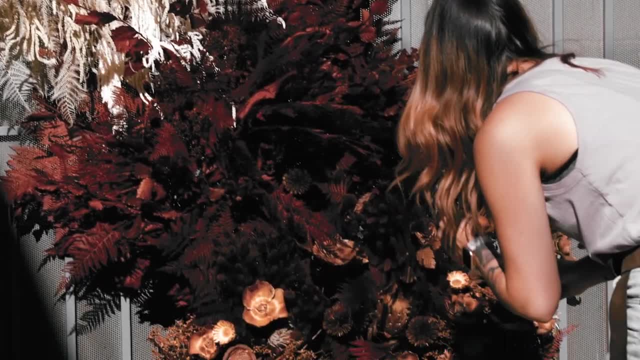 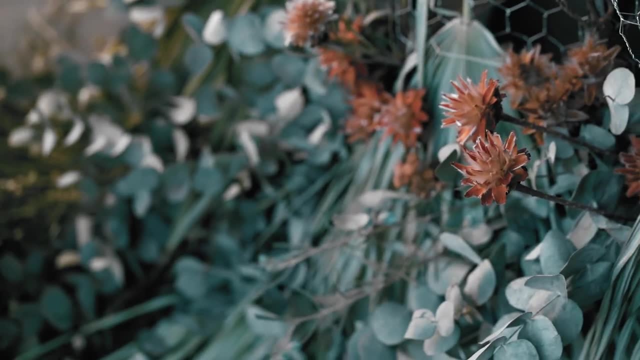 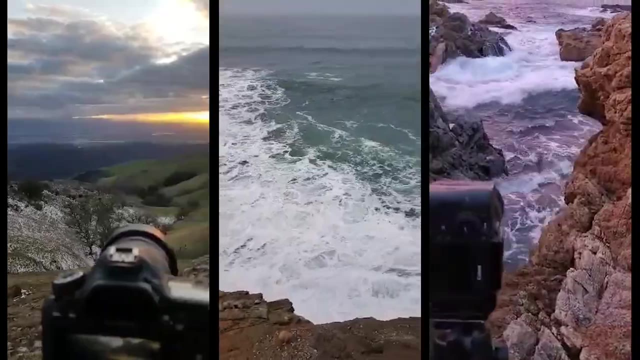 or a designer of any kind, The type of person who plays with that language of light and recognizes which colors complement each other. Photographers are great examples of visually intelligent people. They recognize those moments that are worth capturing, Those moments that are especially beautiful or compelling. 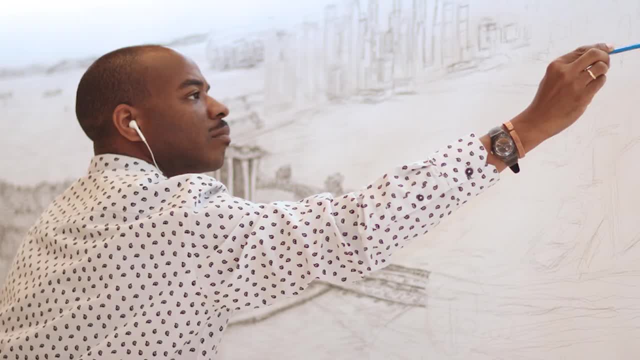 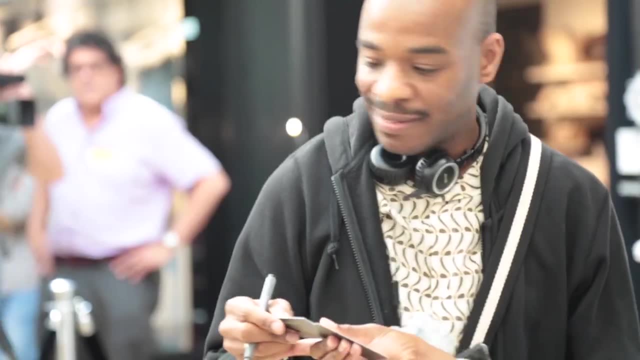 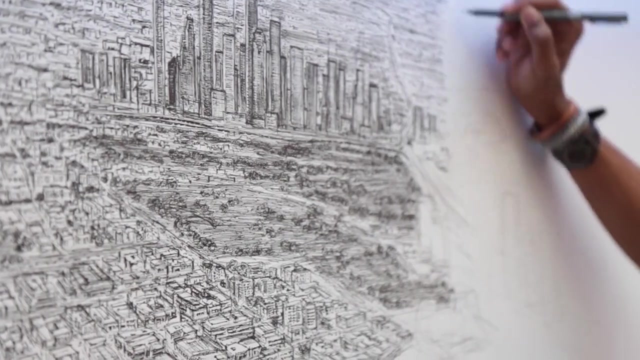 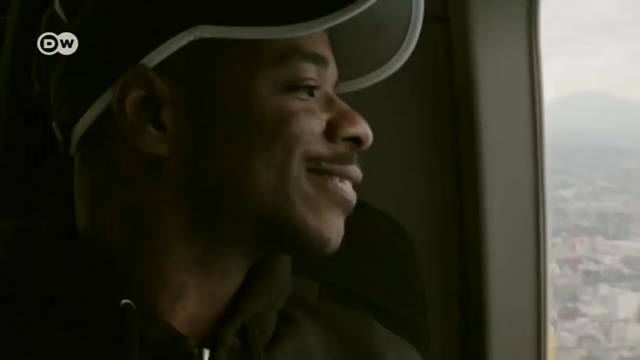 Another example of a genius of visual intelligence is Stephen Wiltshire, who is an artistic autistic savant who became famous for his ability to draw entire cityscapes from memory after seeing them once, And the details are always accurate. In 2001,, Stephen took a helicopter ride over London. 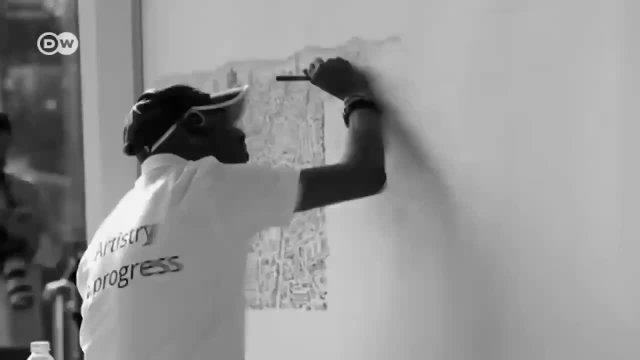 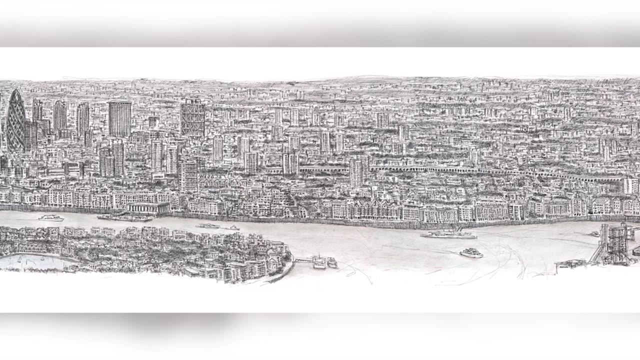 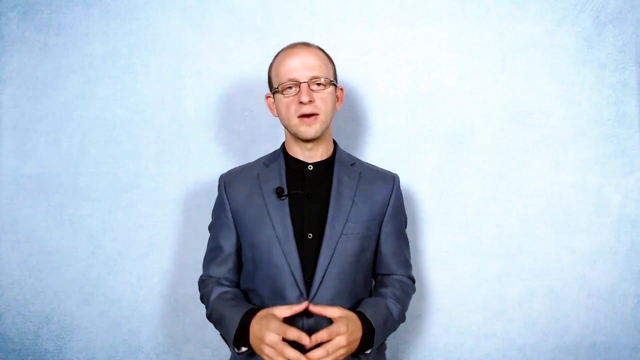 and subsequently completed a detailed and perfectly scaled illustration of a four-square-mile area. His drawing included 12 landmarks and 200 other structures, And every detail was precise. So Akiana Kramarik and Stephen Wiltshire are both geniuses at visual intelligence. 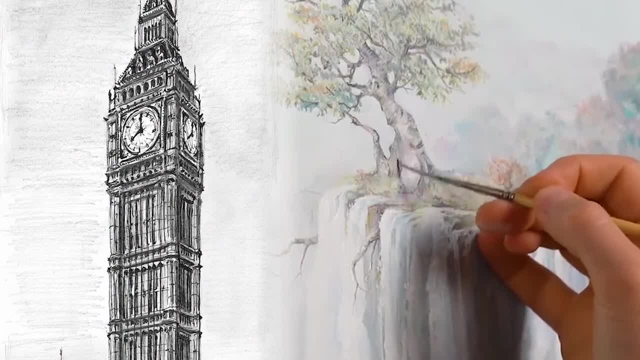 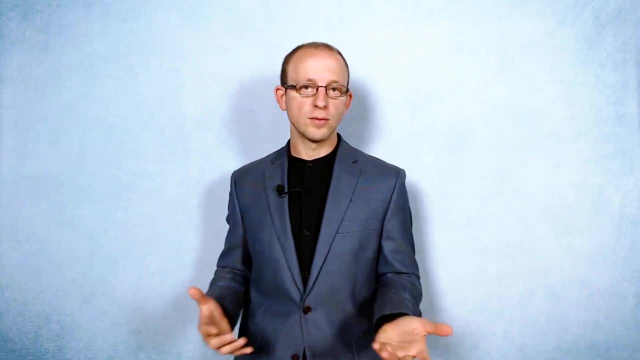 But when you hold their work up next to each other, it doesn't even look all that similar to each other. When we see differences between people who possess the same intelligence, part of the reason for that is the fact that there are many different aspects. 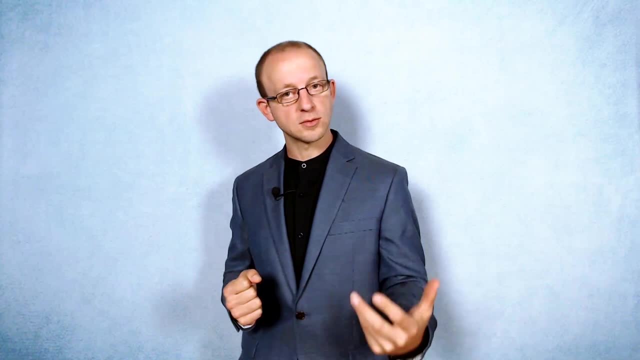 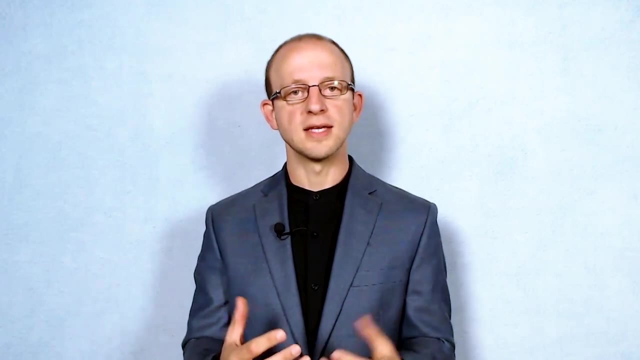 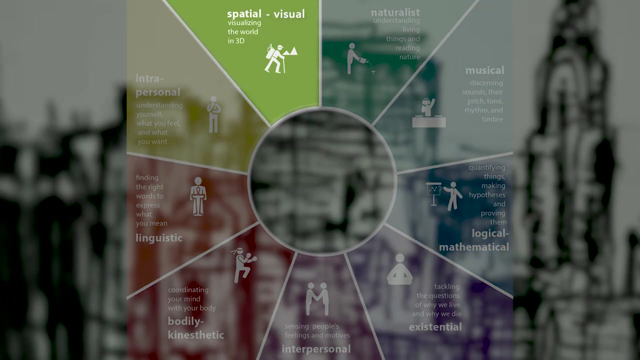 that can be more pronounced in the way that a person expresses that intelligence, But also it relates to what other intelligence the person possesses prominently. So when you look at the mind of Stephen Wiltshire, along with his genius visual intelligence, he is also fueled by a logical, mathematical intelligence. 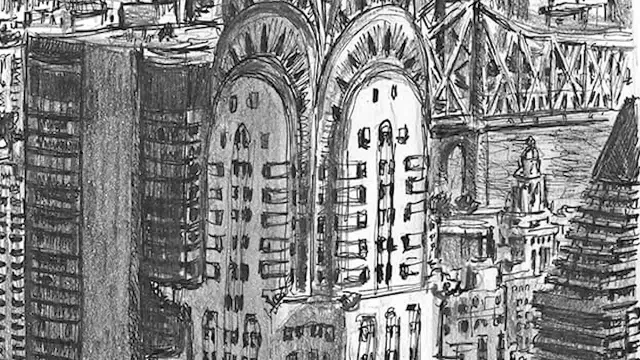 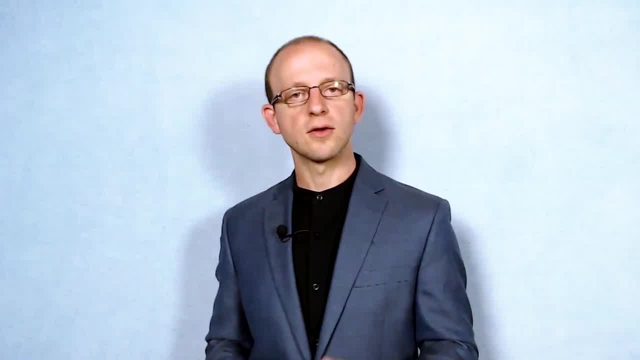 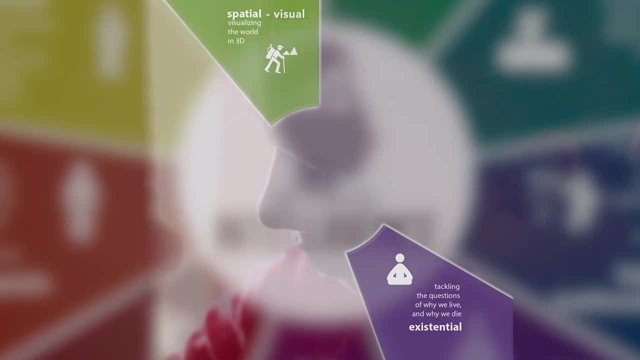 You see this in the way that he draws the number of stories in every building of the cityscapes. he's drawing with precision. In my assessment, Akiana Kramarik is also fueled by existential intelligence. She's just very deep and philosophical. 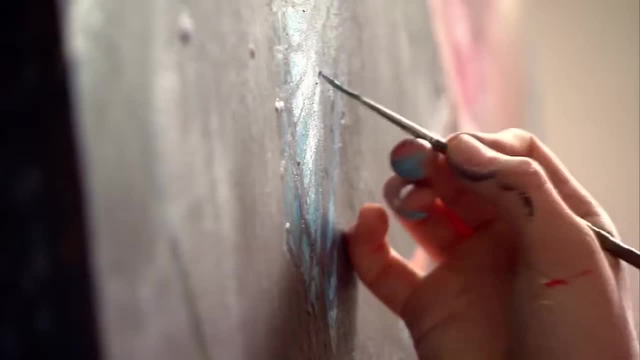 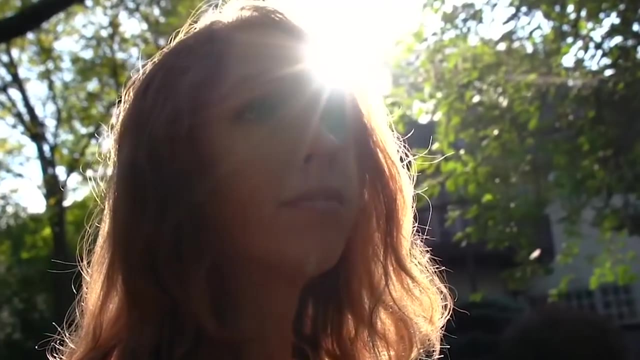 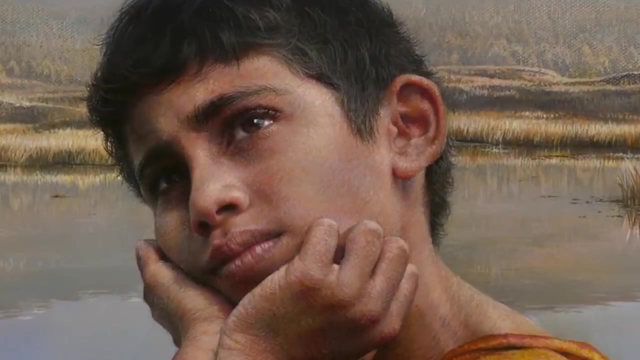 She questions the nature of existence. She contemplates and connects with this higher power that has been inspiring her work from the beginning. As Akiana has blossomed into a woman, the depth and beauty of her art has become utterly profound Among the many ways that we can all become more intelligent. 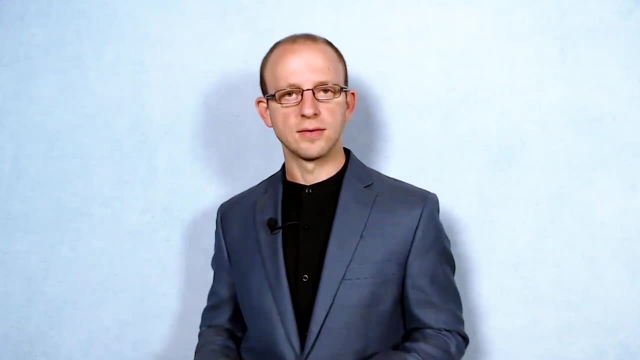 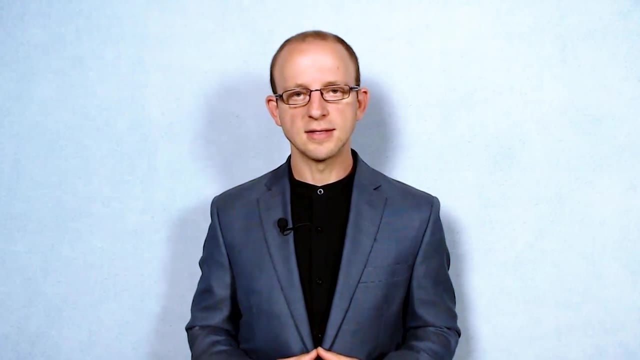 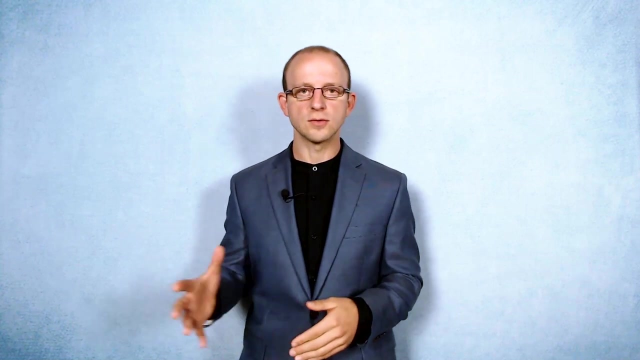 is to take in what geniuses have put out, To recognize the people who are geniuses in the intelligence that you were inspired to cultivate, and study their work. If you're linguistically intelligent and want to be a writer, study the works of genius writers.